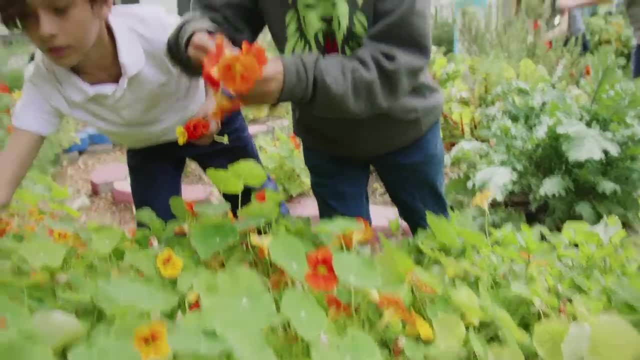 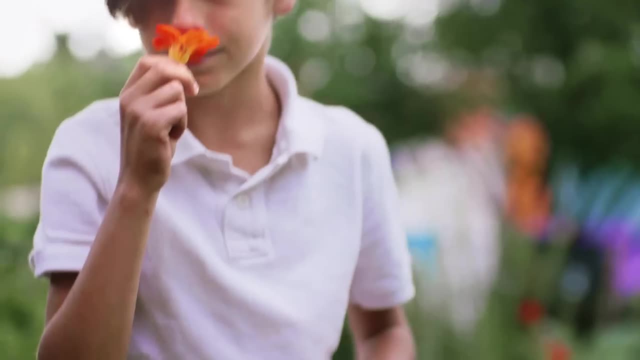 Being in the garden, you're in touch with nature. Oh dude, look at those pink ones. These are edible flowers that you can eat Outside. you're more in the sunlight, with butterflies and different animals. It seems like it's a still life, but everything's moving around. You just can't see it. 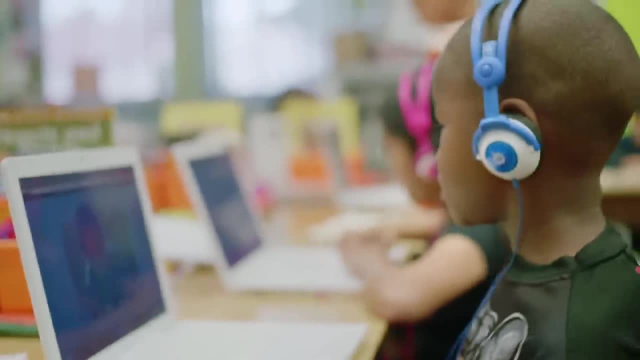 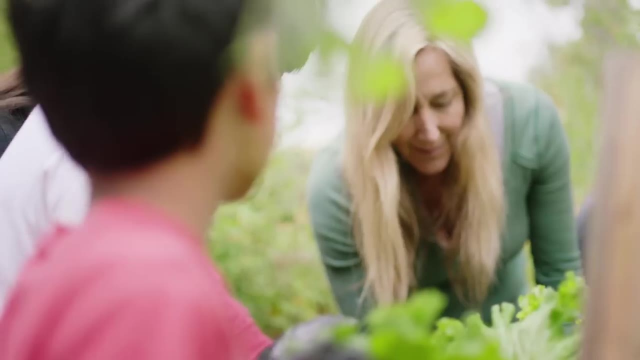 Because we're all absorbed in our electronics and technology nowadays And I think that we should get outside more In school. you just get book smart Here. you get outdoor smart Fruit. Fruit Fruit grows the seed, Fruit grows the seed. 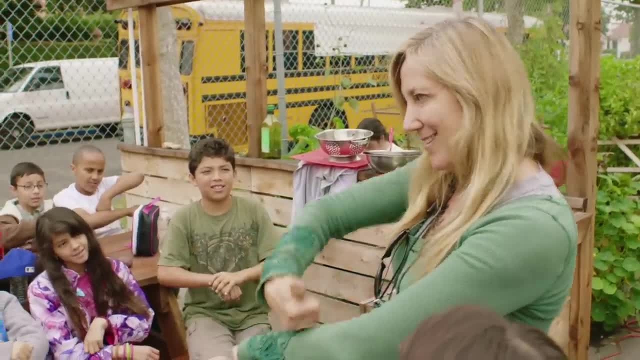 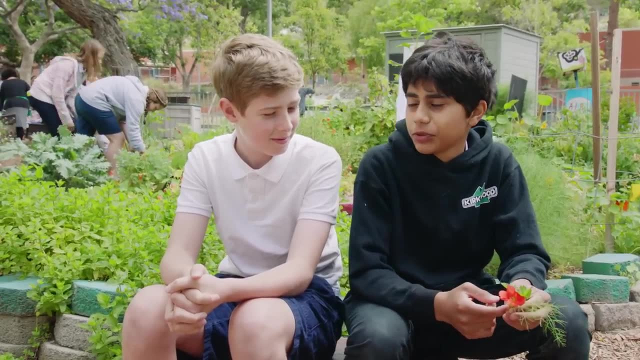 Seed, Seed Back to the earth. Back to the earth, New plant grows, New plant grows. If you're just out here in the woods you forget your snacks, what you gonna do? You gonna eat your foot. No, You're gonna want to make something. 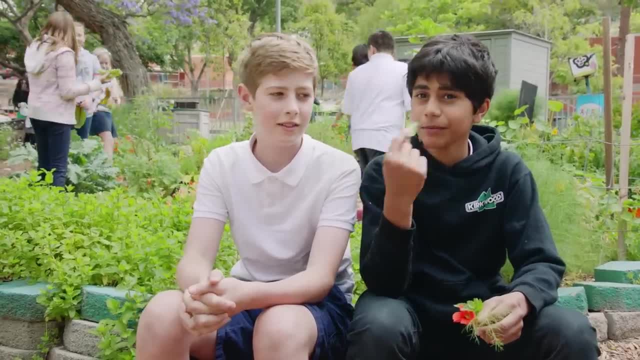 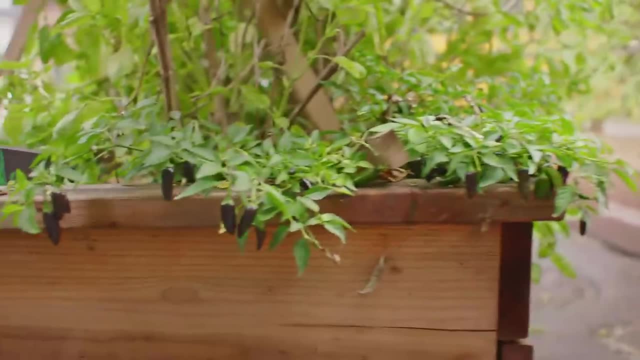 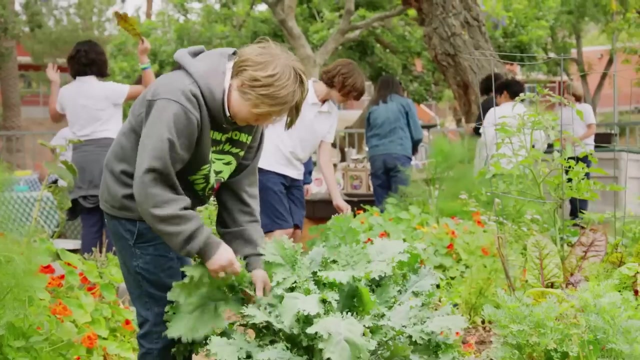 And you also want to know what's edible Mint leaf anyone. We have Tomatoes here. We have strawberries down here. Purple chili peppers. We got jalapeno. We also have kale. These are pecans. Everybody should have a chance to get freshly picked fruits, mangoes, vegetables, peaches, anything. 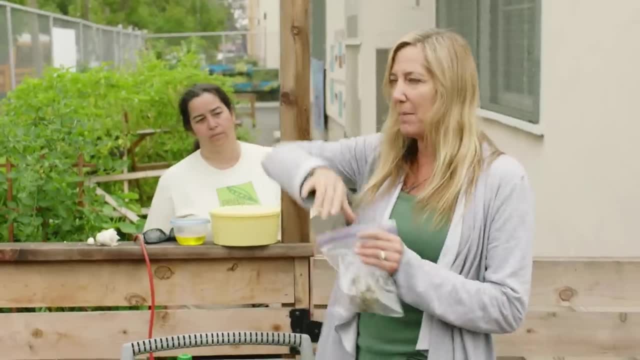 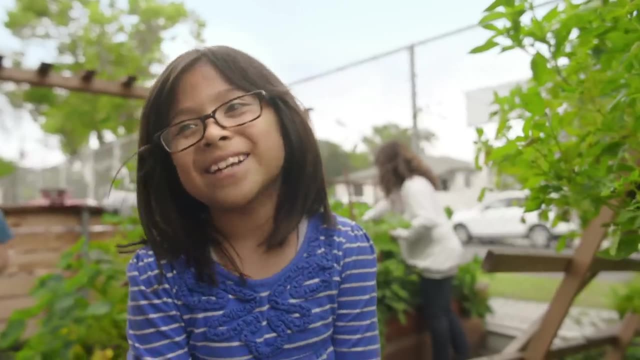 How many of you want to eat artichokes and how many want to make pesto, Pesto, Pesto, Pesto, Pesto. Today we got pesto. We need basil leaves. They give the flavor to the pesto. 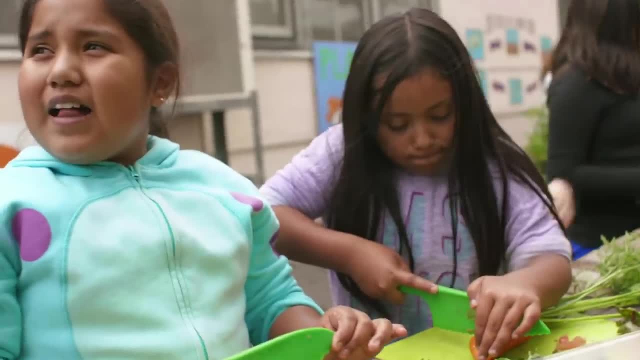 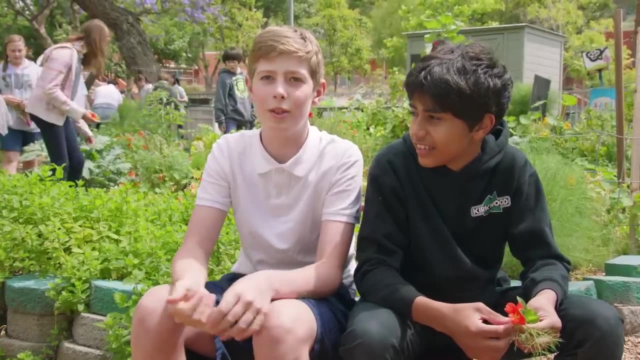 I never really tried them before. We're making a salad, We're just adding a lot of like vegetables Here. I'll do the tomatoes, You do that. I also really like that we get to grow our own plants and that we get to eat them in the end. 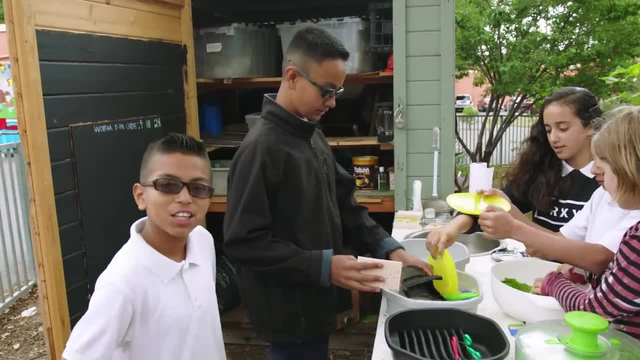 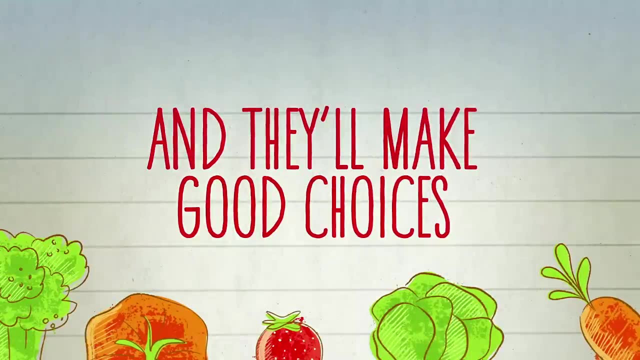 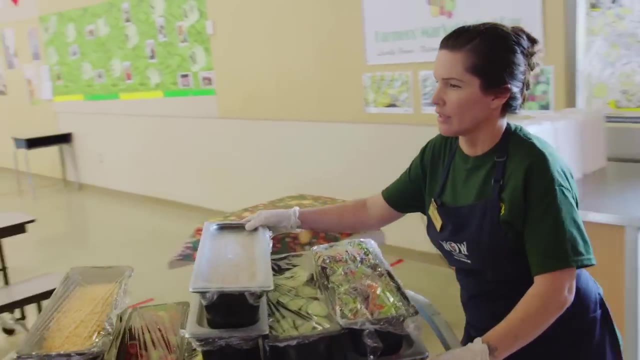 And you actually learn that some foods are actually not that bad when you combine other foods with other things. Pesto, Pesto, Pesto, Pesto. I tried cucumbers at the salad bar for my first time and I really liked them. 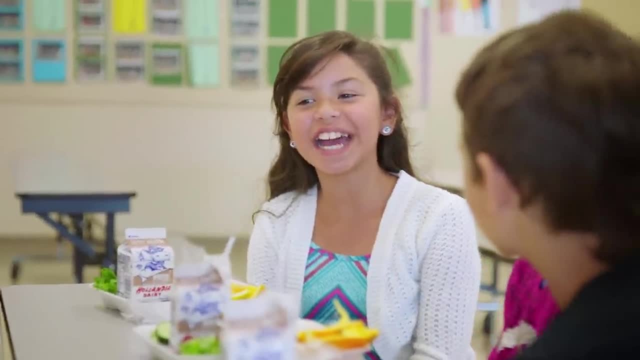 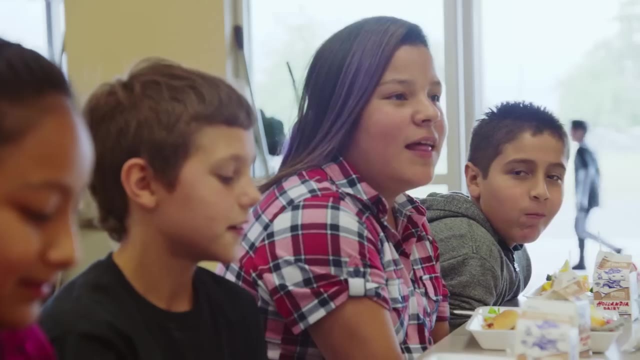 My mom tried feeding me broccoli but I thought it was gross, And then when I came to school I saw my friends eating it, so I grabbed some and ate it and I thought it was good. I like the salad bar because there's many choices to choose from.